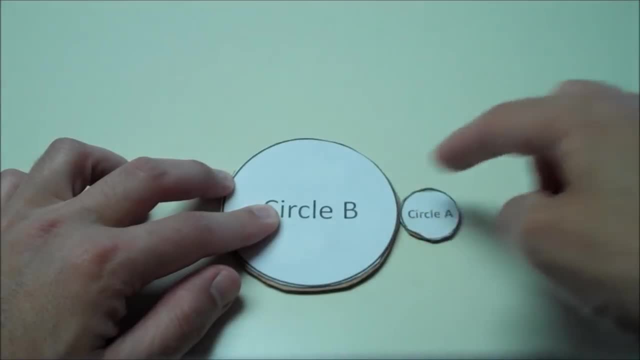 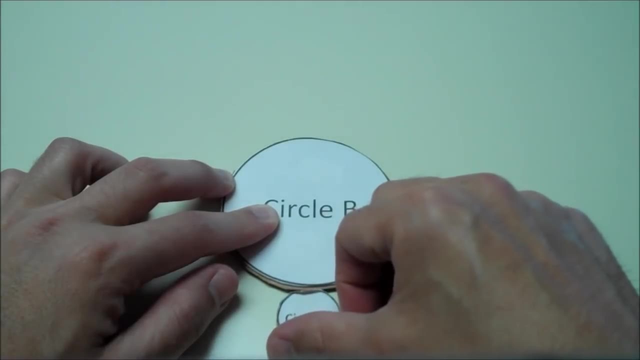 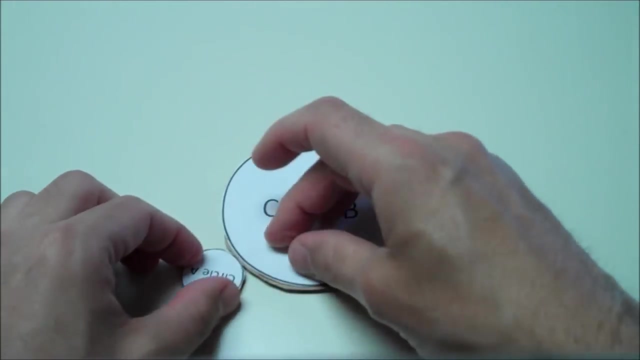 after one quarter of the distance, circle A has already revolved around one time. When we go halfway around circle B, circle A has rolled around a second time. As we continue around we'll see that by 3 fourths of the distance circle A will roll a third time. 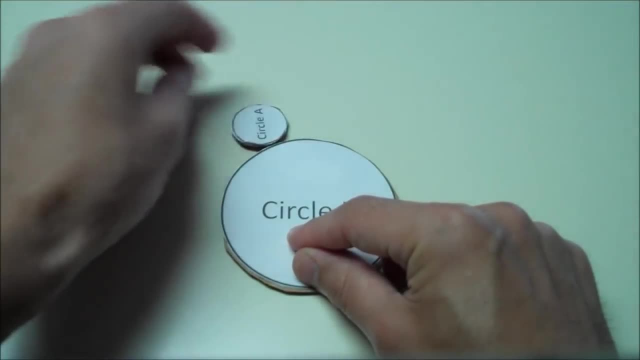 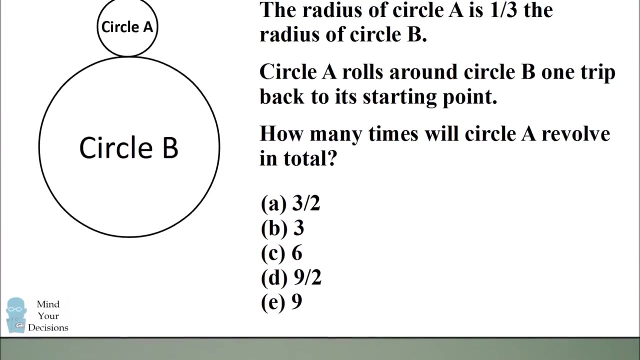 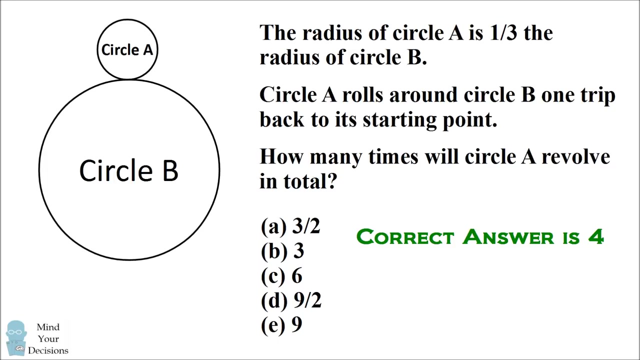 And when we complete the trip, as circle A rolls around, circle B when it completes the trip, this will be a fourth time that circle A has rolled around, So the correct answer is 4.. And they actually made a mistake. They did not include this as the correct answer. 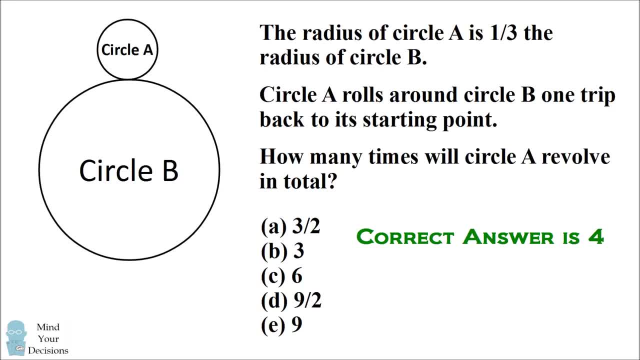 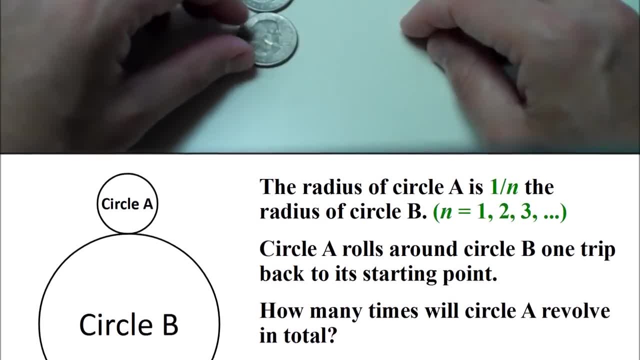 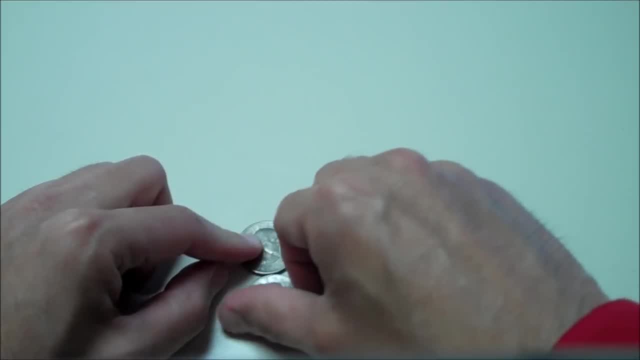 They forgot to take into account that circle A is revolving around circle B and that would have added one more trip around. Let's try and solve this problem in general. Imagine having two coins of equal circumference. You would think the answer might be 1.. 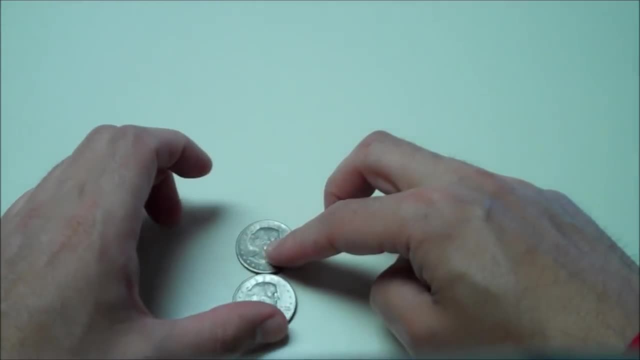 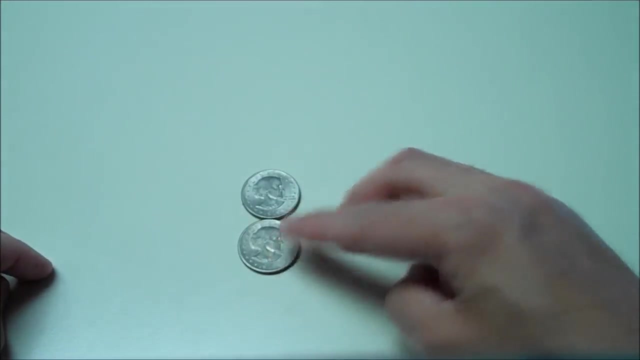 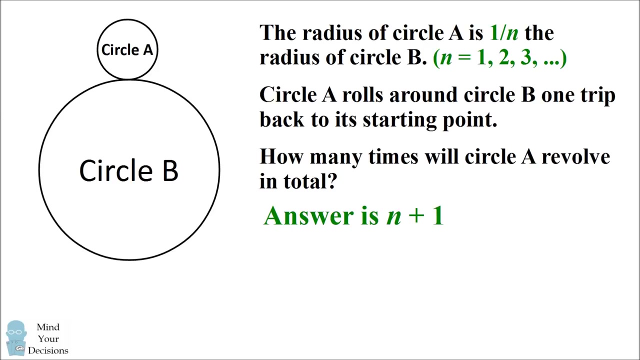 But you see that when the coin rolls around halfway, it's already rolled around one time. When it rolls around the remaining distance, it will roll around a second time. So we can solve this problem and we'll see. the correct answer is that circle A will roll around n plus 1 times. 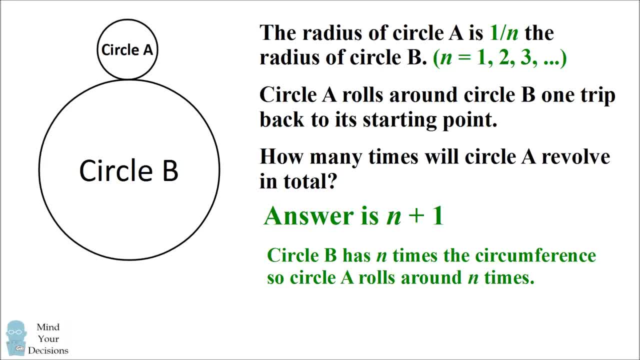 The reason is that circle B has n times the circumference and that will account for n times that the circle A revolves around itself. But then we will also get one more revolution, because circle A is also revolving around the center of circle B. So the correct answer is n plus 1.. 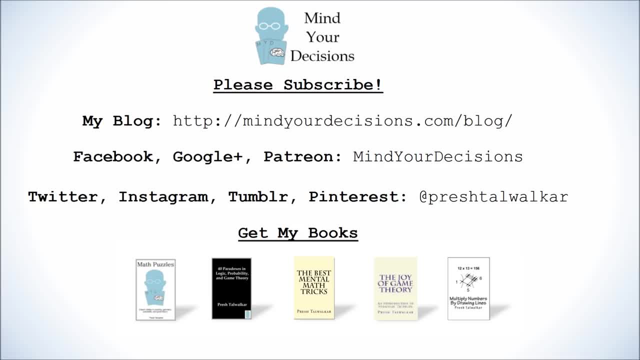 It's a pretty interesting problem. I hope you liked the video. Please subscribe to my channel. I make videos on math and game theory. You can catch me on my blog Mind Your Decisions, which you can follow on Facebook, Google+ and Patreon. 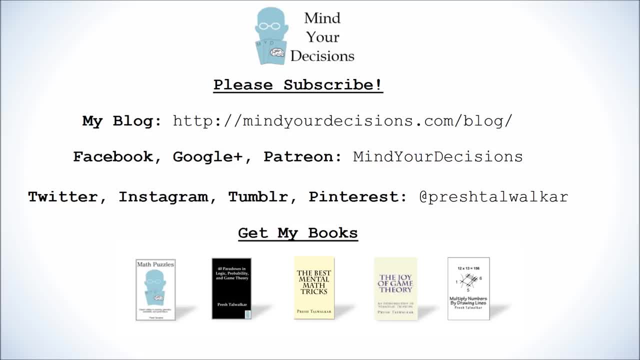 You can also catch me at Presh Talwalkar on social media And, if you liked the video, please check out my books. I've provided links in the video description. Thanks for watching. 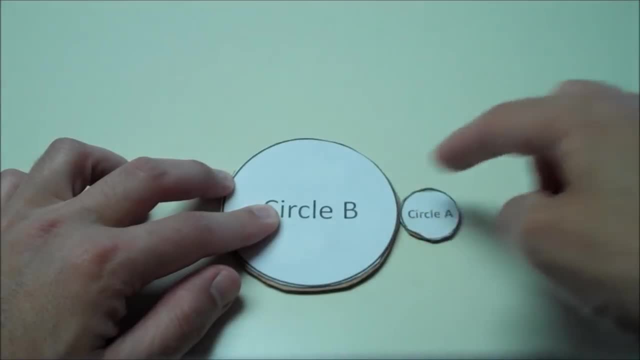 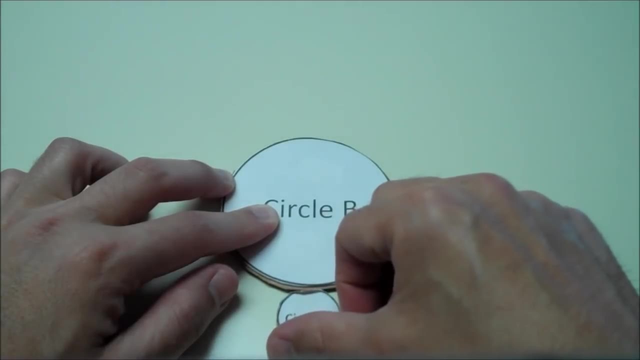 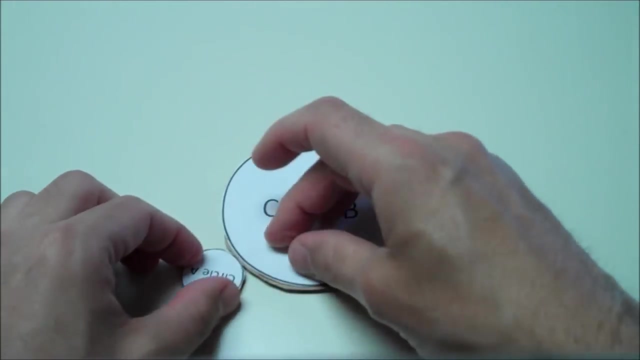 after one quarter of the distance, circle A has already revolved around one time. When we go halfway around circle B, circle A has rolled around a second time. As we continue around we'll see that by 3 fourths of the distance circle A will roll a third time. 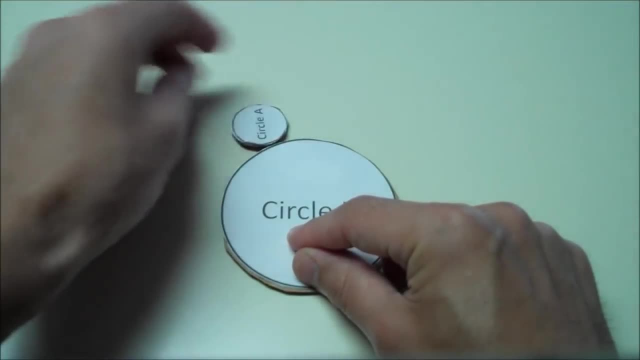 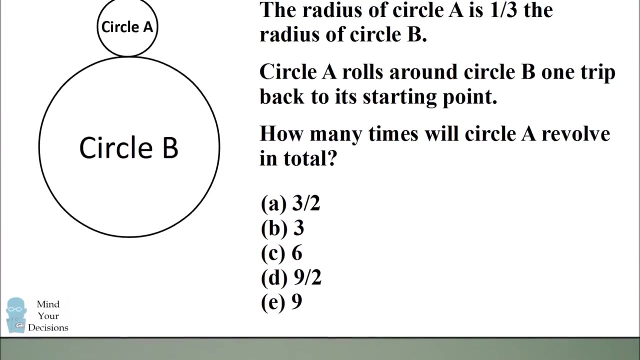 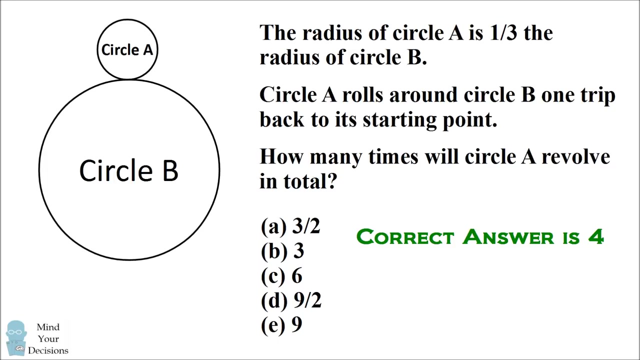 And when we complete the trip, as circle A rolls around, circle B when it completes the trip, this will be a fourth time that circle A has rolled around, So the correct answer is 4.. And they actually made a mistake. They did not include this as the correct answer. 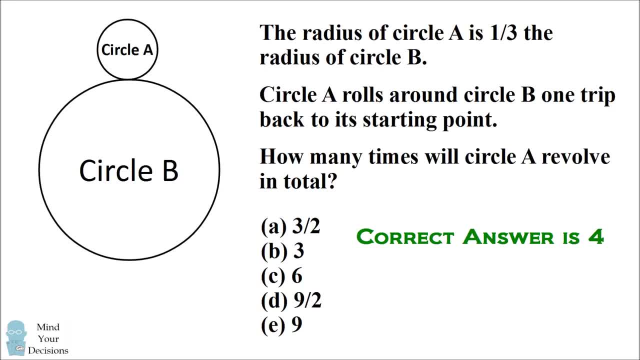 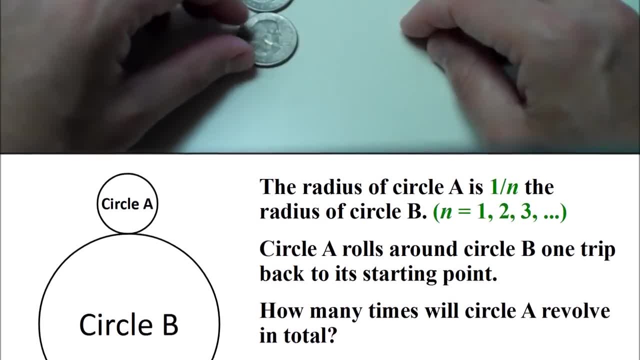 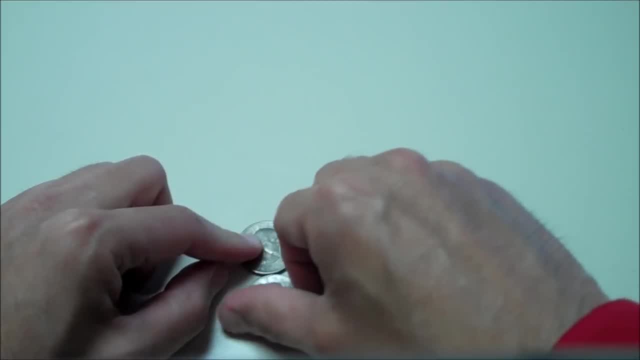 They forgot to take into account that circle A is revolving around circle B and that would have added one more trip around. Let's try and solve this problem in general. Imagine having two coins of equal circumference. You would think the answer might be 1.. 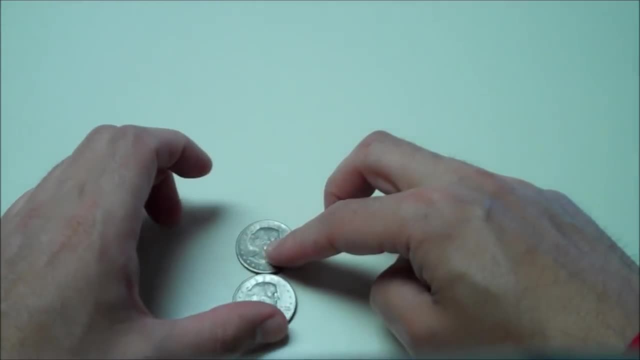 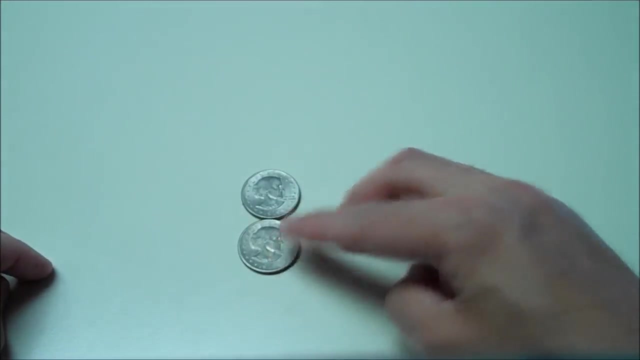 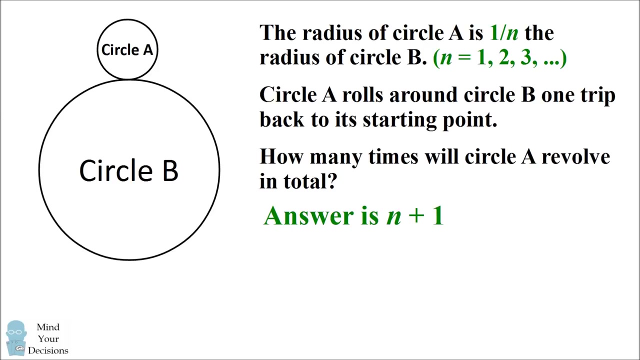 But you see that when the coin rolls around halfway, it's already rolled around one time. When it rolls around the remaining distance, it will roll around a second time. So we can solve this problem and we'll see. the correct answer is that circle A will roll around n plus 1 times. 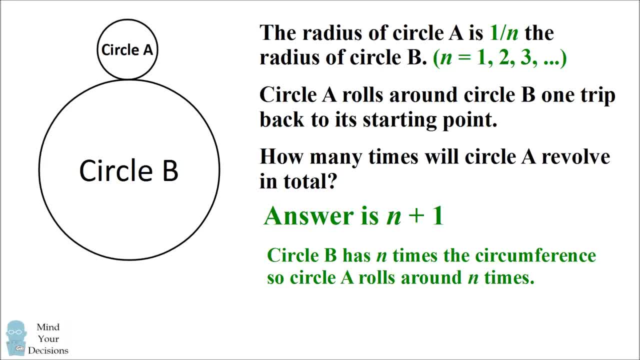 The reason is that circle B has n times the circumference and that will account for n times that the circle A revolves around itself. But then we will also get one more revolution, because circle A is also revolving around the center of circle B. So the correct answer is n plus 1.. 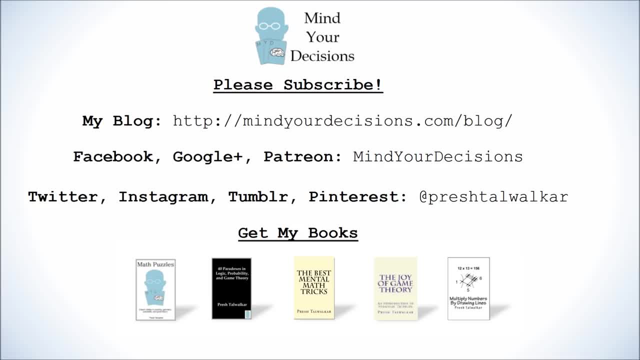 It's a pretty interesting problem. I hope you liked the video. Please subscribe to my channel. I make videos on math and game theory. You can catch me on my blog Mind Your Decisions, which you can follow on Facebook, Google+ and Patreon. 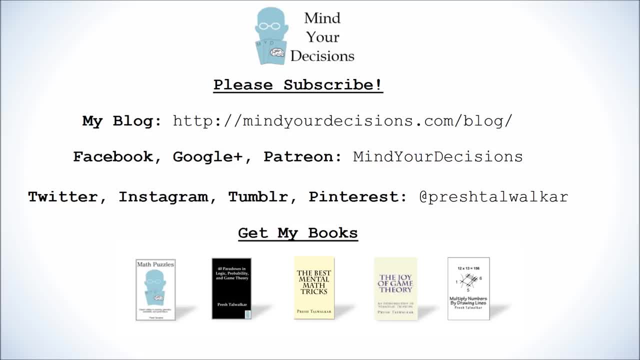 You can also catch me at Presh Talwalkar on social media And, if you liked the video, please check out my books. I've provided links in the video description. Thanks for watching.